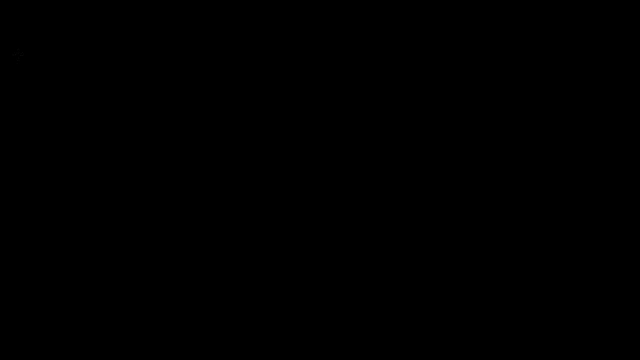 We now have the tools, I think, to understand the idea of a linear subspace of Rn. Let me write that down. I'll just always call it a subspace of Rn. Everything we're doing is linear Subspace of Rn. 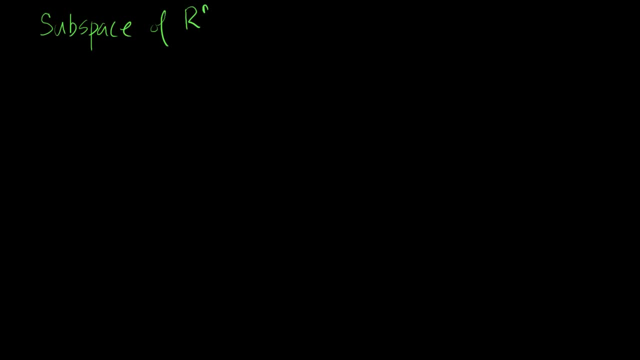 I'm going to make a definition here. I'm going to say that a set of vectors, v. so v is some subset of vectors, subset, some subset of Rn. So we already said Rn. when we think about it, it's really. 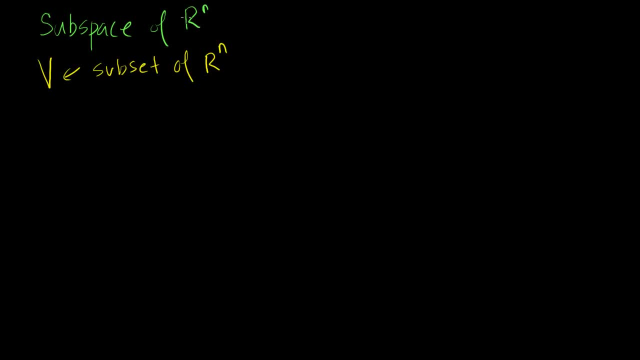 just an infinitely large set of vectors, where each of those vectors have n components. So I'm going to not formally define it, but this is just a set of vectors. I mean, sometimes we visualize it as multidimensional space and all of that. but if we wanted to be just as abstract. 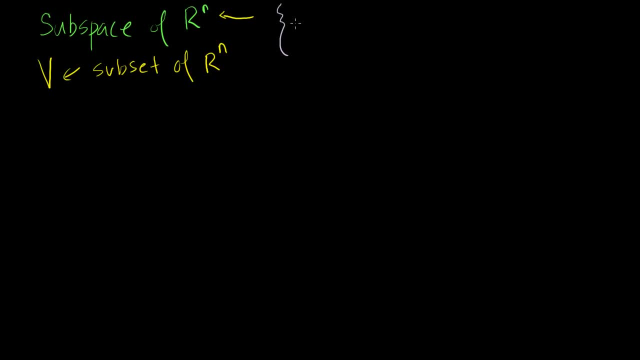 about it as possible. It's just all the set. it's the set of all of the. you know we could call it x1,, x2, all the way to xn, where each of these, where each of the xi's are a member of the real. 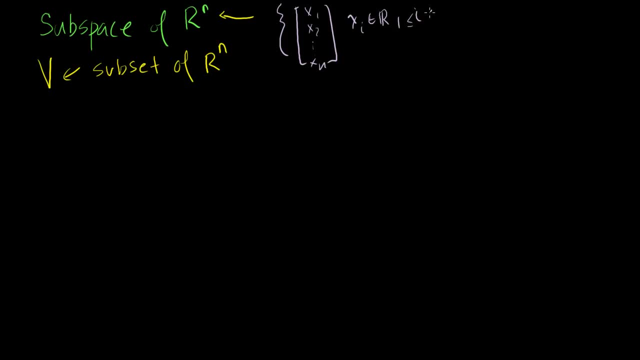 numbers for i's, for all of the i's. That was our definition of Rn. It's just a huge set of vectors, an infinitely large set of vectors. v I'm calling that. I'm going to call that a subset of Rn. 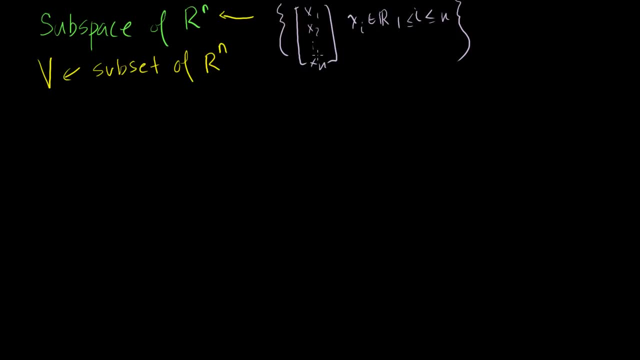 which means it's just subspace, Subset of Rn, Subset of Rn. So some you know it could be all of these vectors and I'll talk about it in a second, or it could be some subset of these vectors. 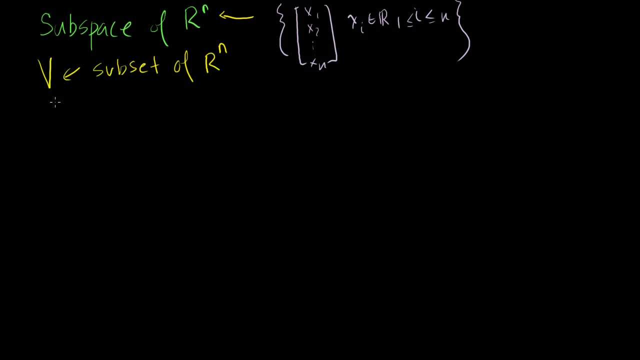 Maybe it's all of them, but one particular vector, And in order for this v to be a subspace, so I'm already saying it's a subset of Rn. So if I were to you know, maybe this will help you. 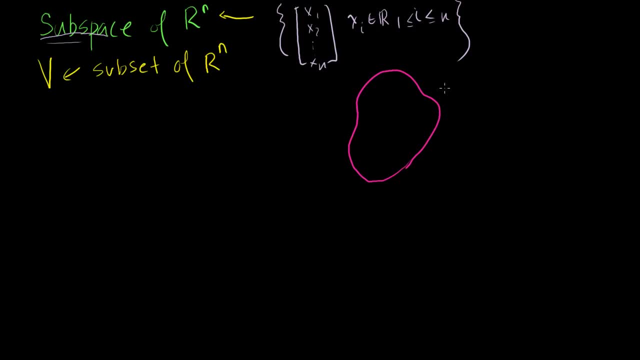 If I draw all of Rn here as this big blob. So these are all of the vectors that are in Rn. v is some subset of it. It could be all of Rn and I'll show that in a second. But let's just call it, let's just say this is v. 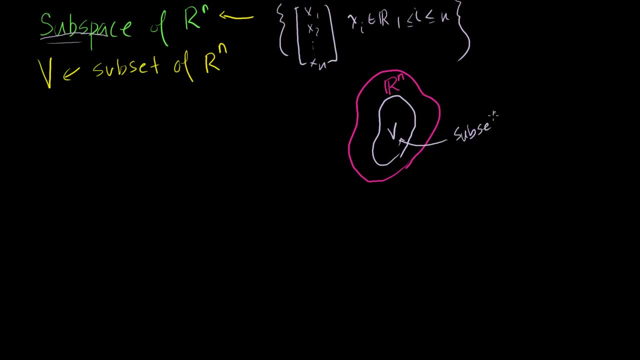 v is a subset of vectors. Now, in order for v to be a subspace- and this is a definition in order- if v is a subspace or a linear subspace of Rn, this means this is my definition, this. 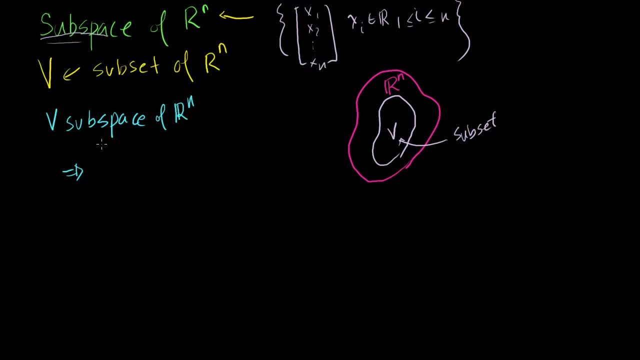 means three things. This means that v contains the 0 vector, v contains- I'll do it really- This is 0 vector, Or you could. you know this is equal to 0, and you have n 0's. 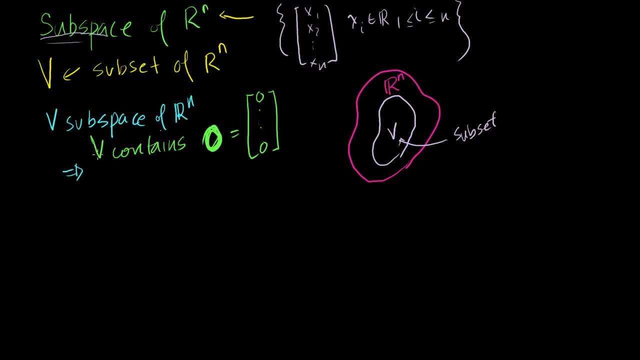 So v contains the 0 vector. This is a big v right there, If we have some vector x in v, So let me write this: So it was x. If my vector x is in, v Is in, Is in. if x is one of these vectors that's included in my v, then 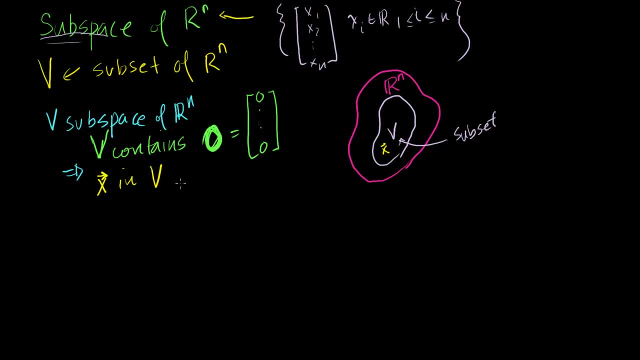 when I multiply x times any member of the reals. so if x is in v, then if v is a subspace of Rn, then x times any scalar is also in v. This has to be the case And for those of you who are familiar with the term, this 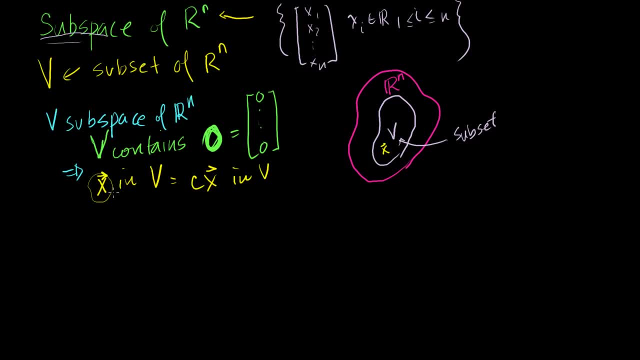 term is called closure. If I have any element of a set, and this is closure under multiplication, Let me write that down into a new color. This is closure under scalar multiplication, And that's just a fancy way of saying: look, if I take some. 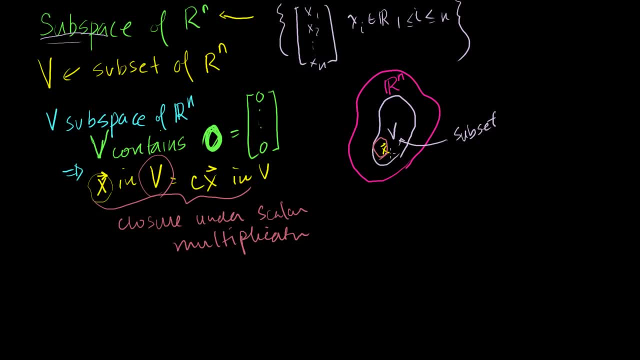 member of my set and I multiply it by some scalar. I'm still going to be in my set If I multiply it by some scalar and I end up outside of my set if I ended up with some other vector, that's not. 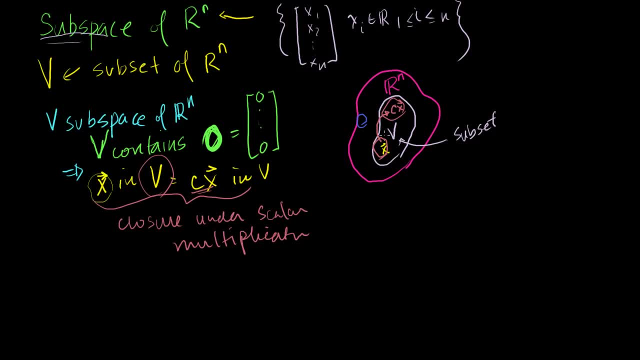 included in my subset, then this wouldn't be a subspace. In order for it to be a subspace, if I multiply any vector in my subset by a real scalar, I'm defining the subspace over real numbers. if I multiply it by any real 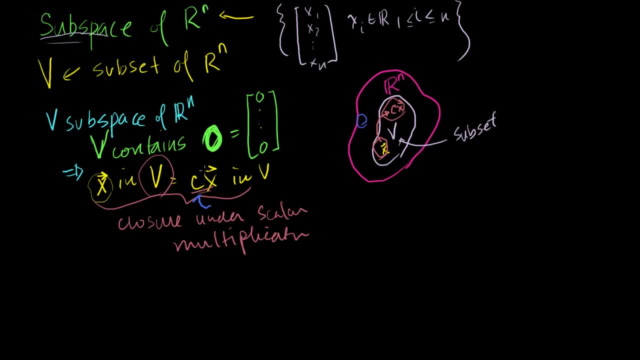 number, I should also get another member of this subset. So this is one of the requirements. And then the other requirement is: if I take two vectors in my, let's say, I have vector A- it's in here and I have vector B in here. 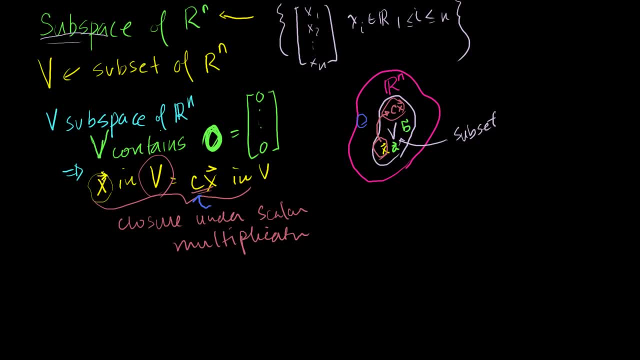 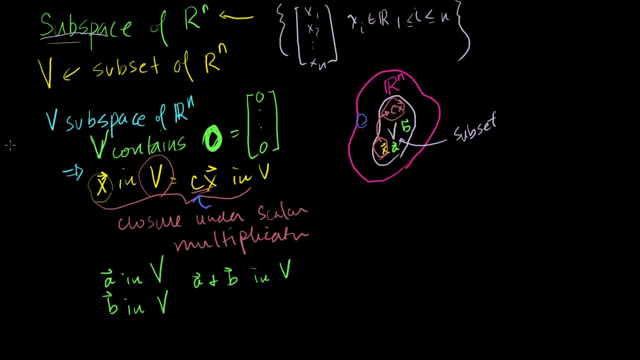 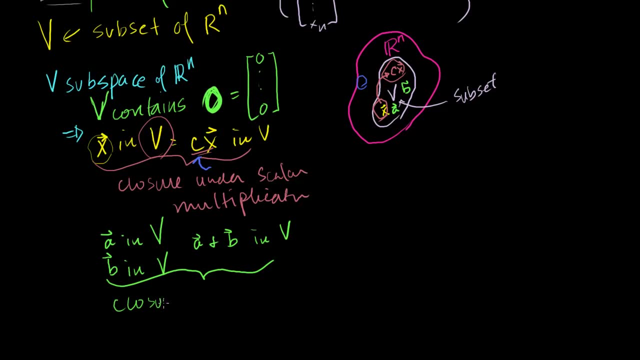 Then if V is a subspace of Rn, that tells me that A and B must be in my set, V must be in V as well. So this is closure under addition. Let me write that down: Closure under addition- Once again, just a very fancy way of saying. look, if you. 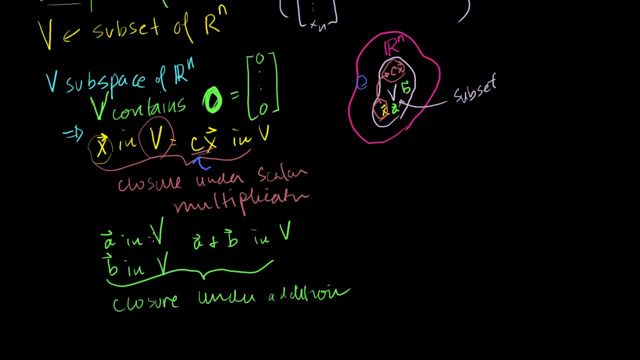 give me two elements that's in my subset and if I add them to each other- and these could be any two arbitrary elements in my subset and I add them to each other, I'm going to get another element in my subset. That's what closure under addition means. 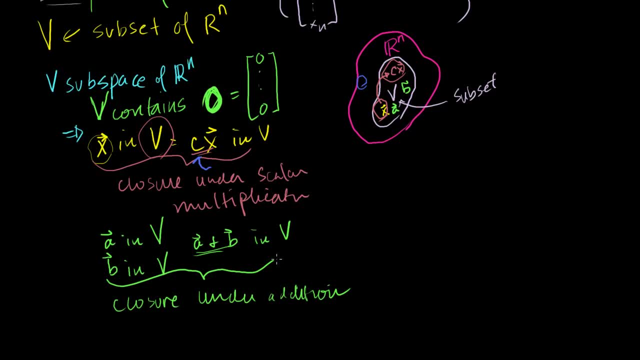 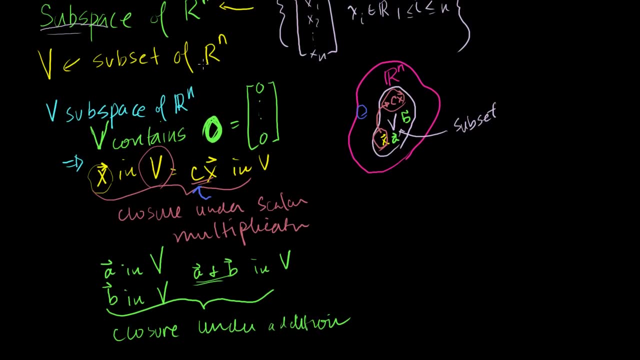 That when you add two vectors in your set, you still end up with another vector in your set. You don't somehow end up with a vector that's outside of your set. So if I have a subset of Rn, so some subset of vectors of. 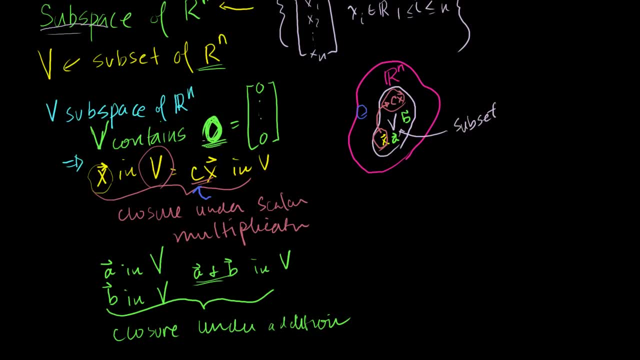 Rn that contains the 0 vector and it's closed under multiplication and addition. then I have a subspace. So subspace implies all of these things, and all of these things imply a subspace. This is the definition of a subspace. 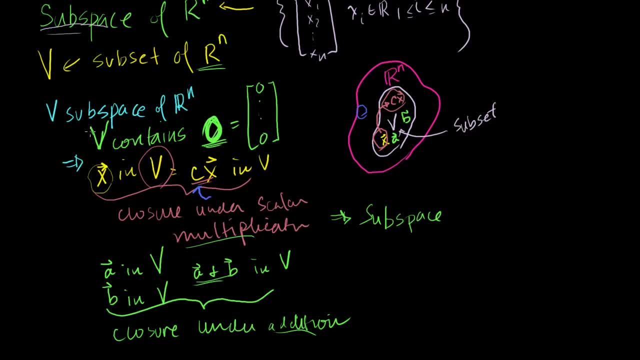 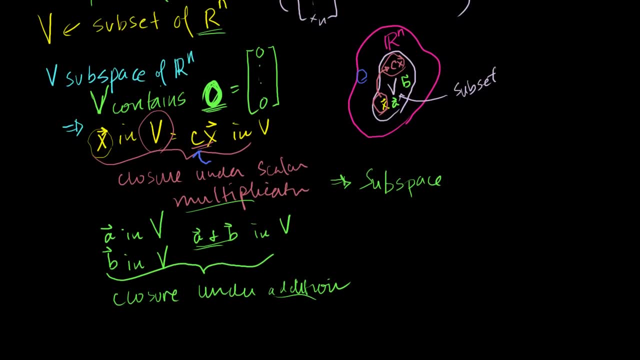 Now this might seem all abstract to you right now. so let's do a couple of examples, And I don't know if the examples will make it any more concrete, but I think if we do it enough you'll kind of get the intuitive sense of what a space implies. 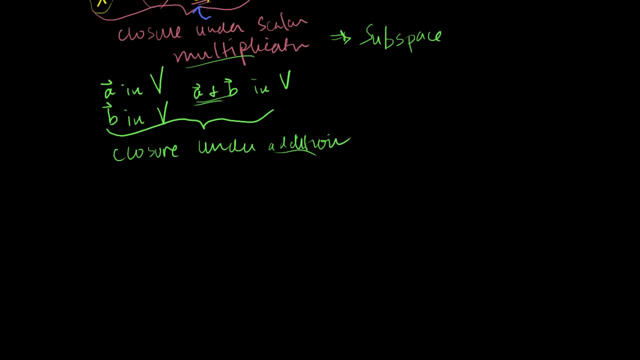 Let me just do some examples because I want to stay relatively mathematically formal. So let's just say I have the almost trivially basic set, Let's say my set of vectors. I only have one vector in it and I have the 0 vector. 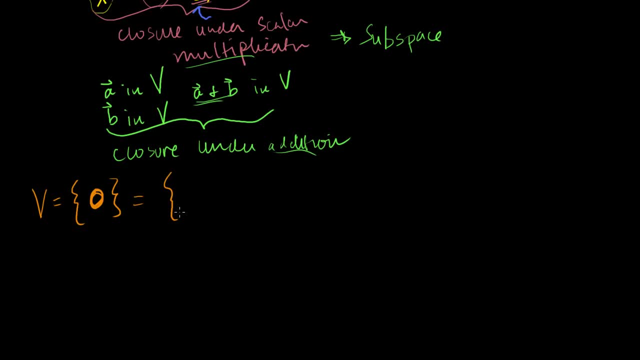 So I'll just do a really bold 0 there, Or I could write it like this: The only vector in my set is the 0 vector, And let's say we're talking about R3.. So let's say, my 0 vector in R3 looks like that: 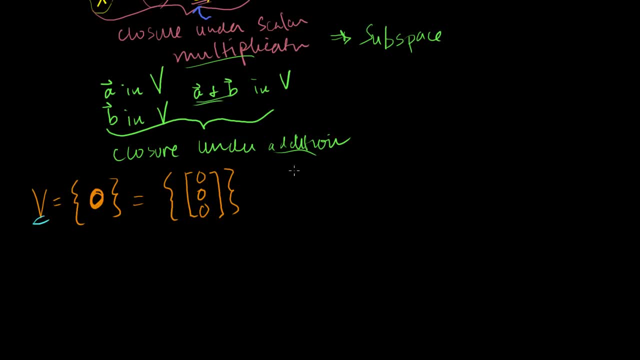 So what I want to know is: is my set v a subspace of R3.. Well, in order for it to be a subspace, three conditions: It has to contain the 0 vector. Well, the only thing it does contain is the 0 vector. 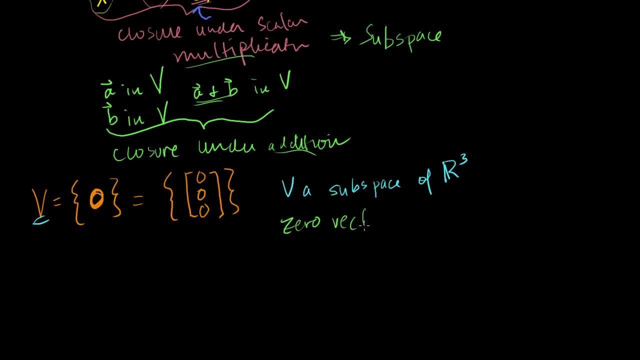 So it definitely contains the 0 vector. So 0 vector check. Now is it closed under multiplication. So that means if I take any member of the set, there's only one of them and I multiply it by any scalar. I. 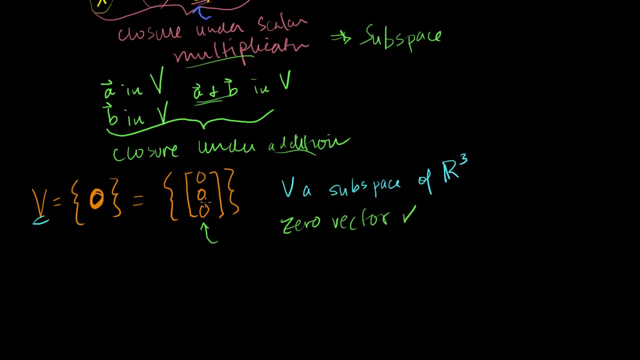 should get another member of the set, Or I should get maybe itself. So let's see, there's only one member of the set, So the one member of the set is the 0 vector. If I multiply it times any scalar, what am I going to get? 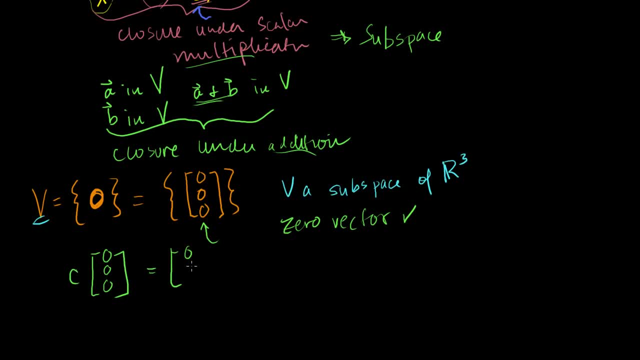 I'm going to get c times 0,, which is 0,, c times 0,, which is 0, and c times 0. So I'm going to get its only member, But it is closed. So it is closed under multiplication. 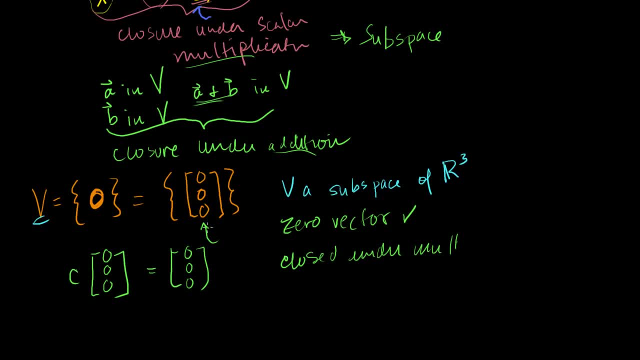 You can multiply this one vector times any scalar and you're just going to get this vector again, So you're going to end up being in your 0 vector. So that's a check. Now is it closed under addition: Well, clearly, if I add any member of this set to itself. 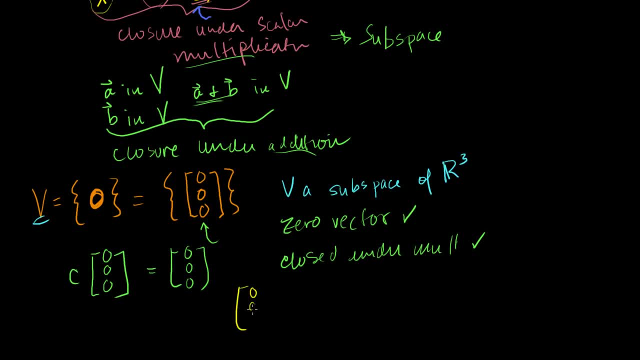 or I mean there's only one member, or to another member of the set: there's only one option here. If I just add that to that, what do I get? I just get that. I just get it again. So it definitely is closed under addition. 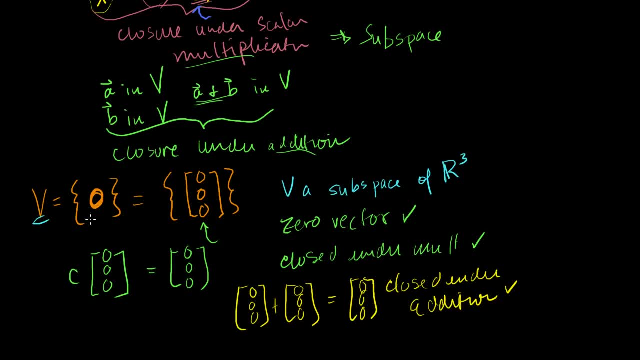 Check. So it does turn out that this trivially basic subset of R3 that just contains the 0 vector, it is a subspace. It is a subspace, Maybe a trivially simple subspace, but it satisfies our constraints of a subspace. 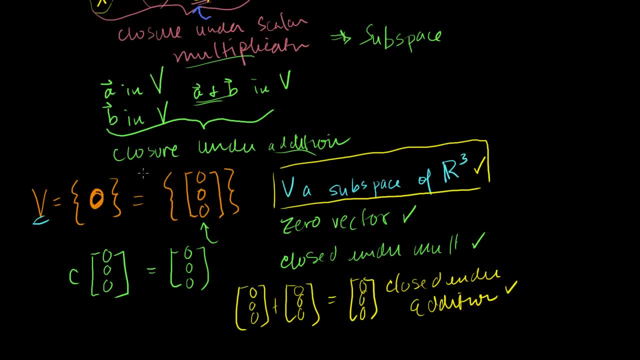 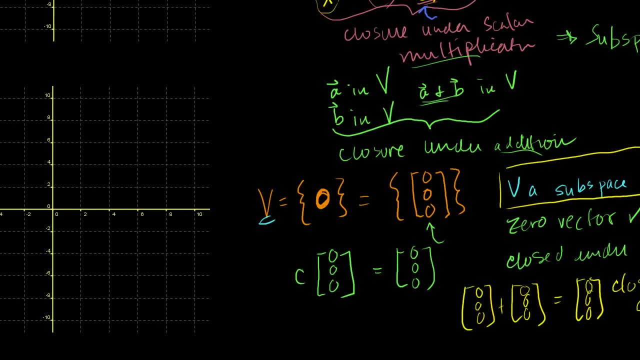 You can't do anything with the vectors in it. that will somehow get you out of that subspace, or at least if you're dealing with scalar multiplication or addition. Now let me do one that. maybe the idea will be a little clearer if I show you an example of something that is. 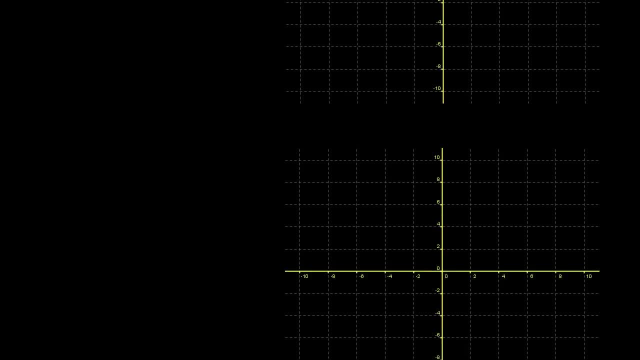 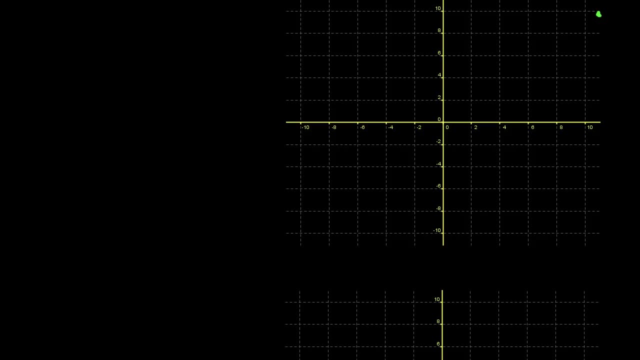 not a subspace. Let me get my coordinate axes over here. So let's say I were to find some subspace, some subset. I don't know whether it's a subspace. Let me call my set S And it equals all the vectors. let me say x1,, x2, that are a. 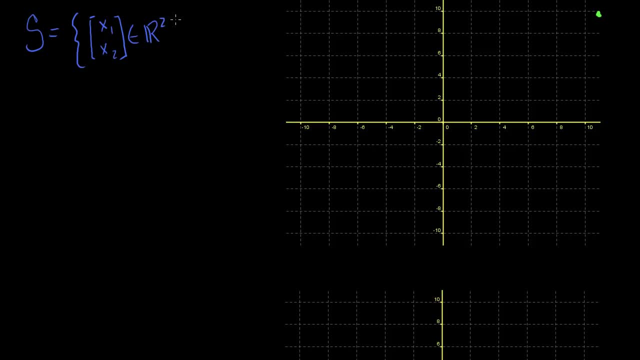 member of R2, such that I'm going to make a little constraint here, Such that x1 is greater than or equal to 0. So it contains all of the vectors in R2 that are at least 0 or greater for the first term. 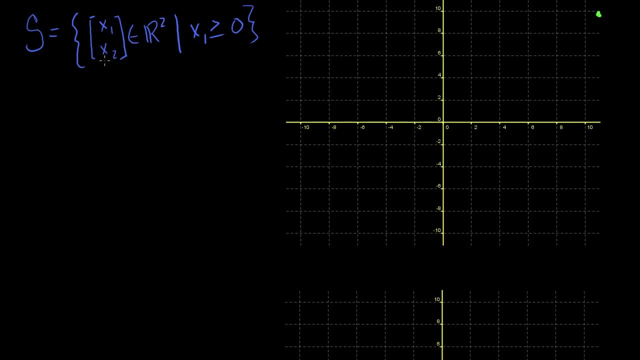 So if we were to graph that here, what do you get? We can move up or down in any direction. So we can go up and down in any direction, but we're constraining ourselves. These are all going to be 0 or greater. 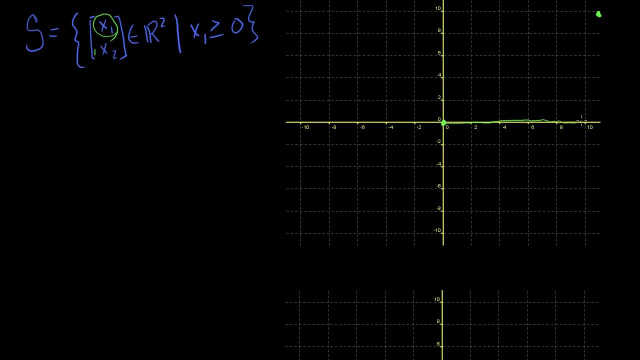 All of these first coordinates are going to be 0 or greater And this one we can go up and down arbitrarily. So essentially, this subset of R2,- R2 is my entire Cartesian plane, But this subset of R2, it'll include the vertical axis. 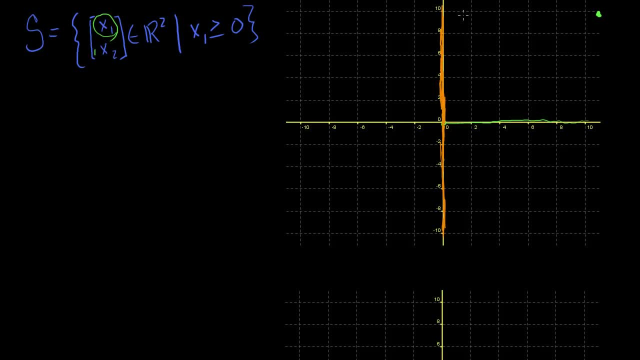 often referred to as the y-axis. It'll include the vertical axis and essentially the first and fourth quadrants, if you remember your quadrant labeling. so that's the first quadrant and that's the fourth quadrant. So my question to you is: is S a subspace of R2?? 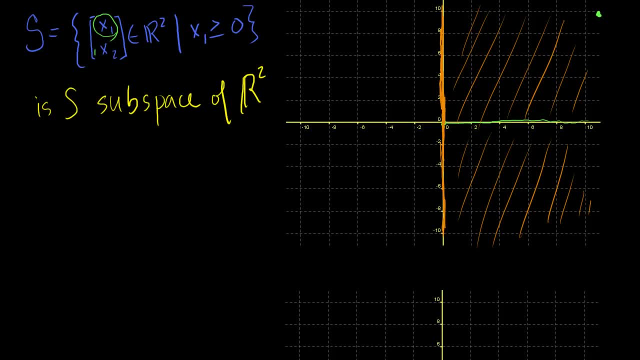 So the first question: does it contain the 0 vector? So, in the case of R2, does it contain 0, 0?? Well, sure, it includes 0, 0's, right there, We included. we said x is greater than or equal to 0. 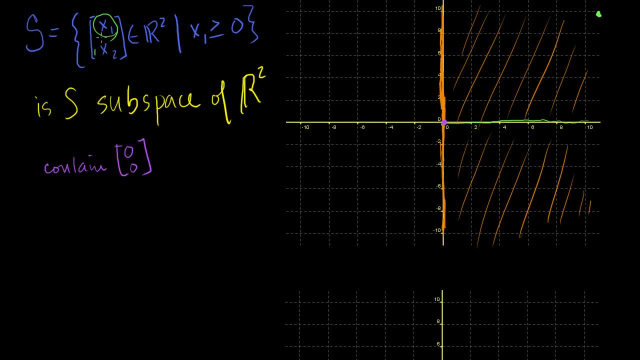 So this could be 0. And obviously there's no constraint on this. So definitely, the 0, 0 vector is definitely contained in our set S. So that is a check. Now let's try another one. If I add any two vectors in the set, is that also going to? 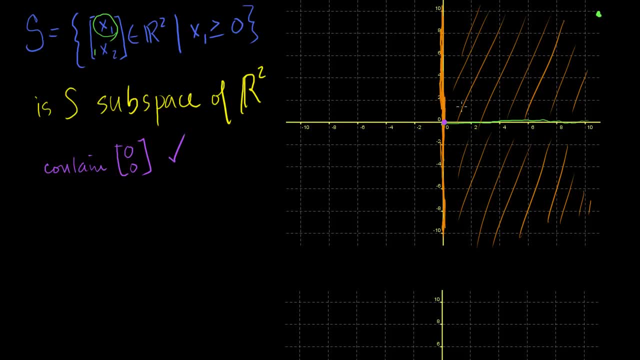 show up in our set. Well, let me just do a couple of examples. Maybe this isn't a proof. Let's see if I add that vector to that vector, what am I going to get If I put this up here? 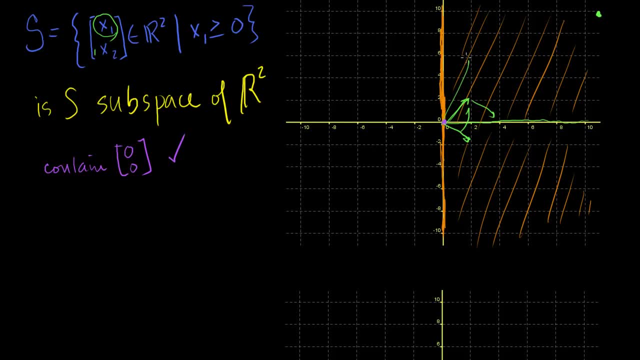 I'm going to get that vector. If I add that vector to that vector, what am I going to get? I could put this one as tail, I would get a vector that looks like that. And if I did it formally, if I add, let's say that I have two. 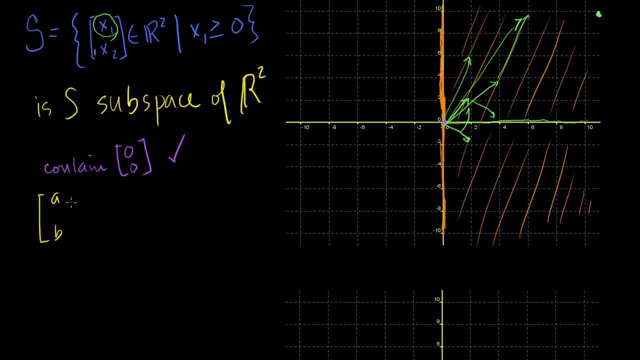 vectors that are a member of our set. So let's say the first one is a- b And I add it to c- d. What do I get? I get a plus c. This was a d over b plus d, So this thing is going to be greater than 0.. 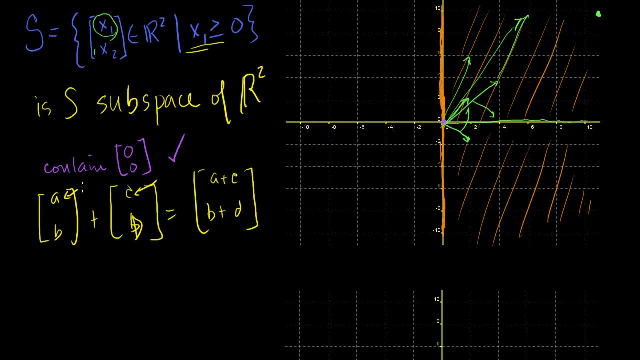 This thing is also going to be greater than 0.. That was my requirement for being in the set. So if both of these are greater than 0 and we add them to each other, this thing is also going to be greater than 0.. 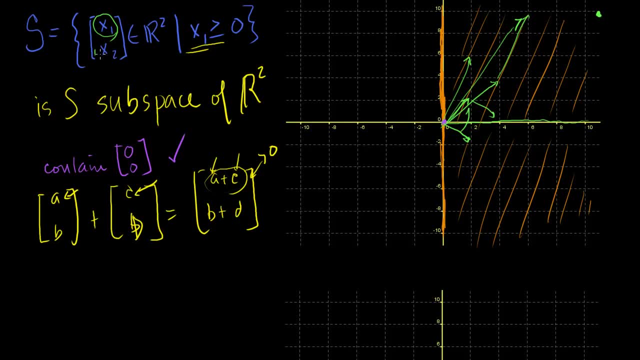 And we don't care with these. These can be anything. I didn't put any constraints on the second component of my vector, So it does seem like it is closed under addition. Now what about scalar multiplication? Let's take a particular case here. 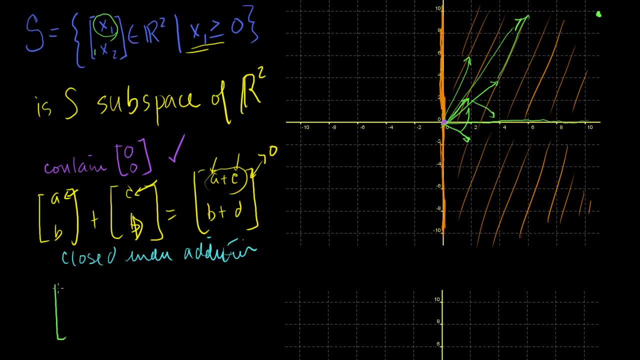 Let's just take my a- b again. I have my vector a- b. Now I can pick any real scalar, Remember any real scalar. what if I just multiply it by minus 1?? So minus 1.. So if I multiply it by minus 1, I get minus a, minus b. 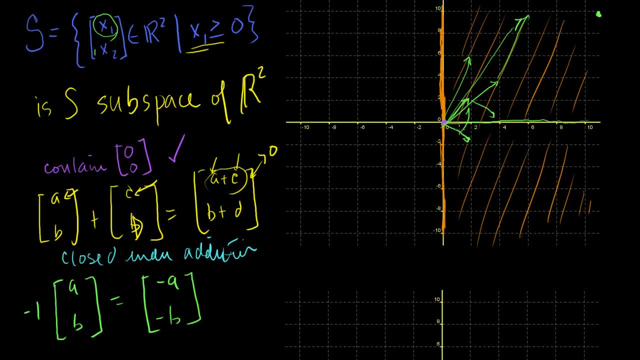 So if I were to draw it visually, if this is, you know, let's say a, b was the vector 2, 4.. So it's like this: When I multiply it by minus 1, what do I get? 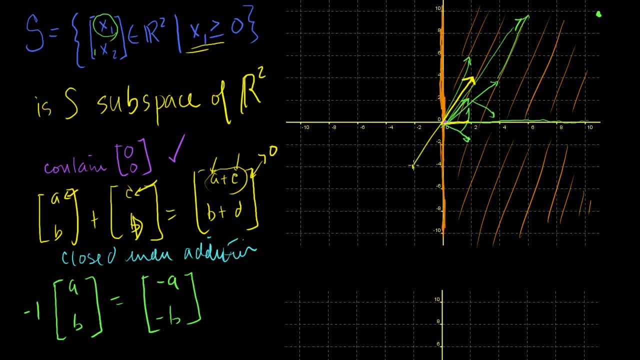 I get minus a, minus b, I get this vector which you can visually clearly see falls out of. if we view these as kind of position vectors, it falls out of our subspace. Or if you just view it, not even visually, if you just do. 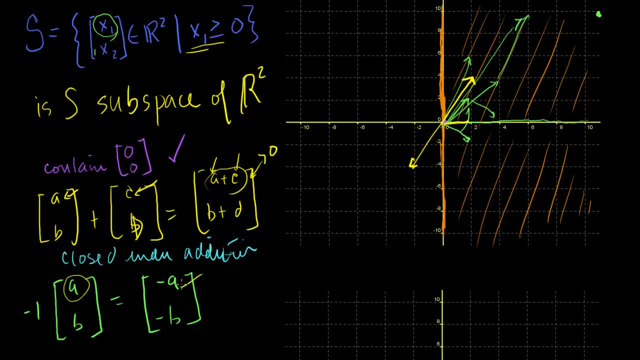 it mathematically Clearly: if this is positive, then this is going to- and let's say that we assume this is positive and definitely not 0. So it's definitely a positive number. So this is definitely going to be a negative number. 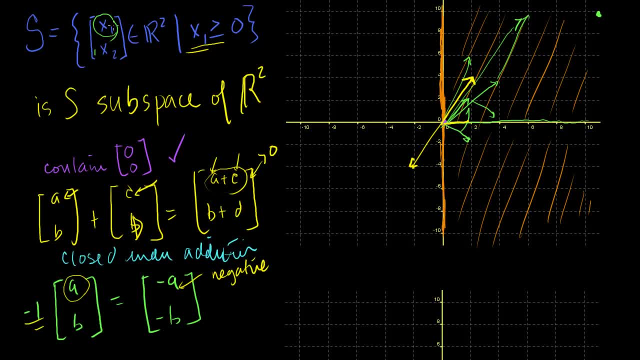 So when we multiply it by negative 1, for really any element of this that doesn't have a 0, there you're going to end up with something that falls out of it. right, This is not a member of the set, Because to be a member of the set, your first component had 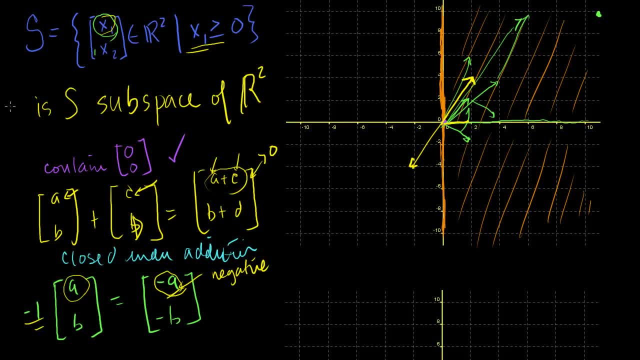 to be greater than 0. This first component is less than 0. So this subspace, So the subset that I drew out here, the subset of R2, is not a subspace because it's not closed under multiplication or 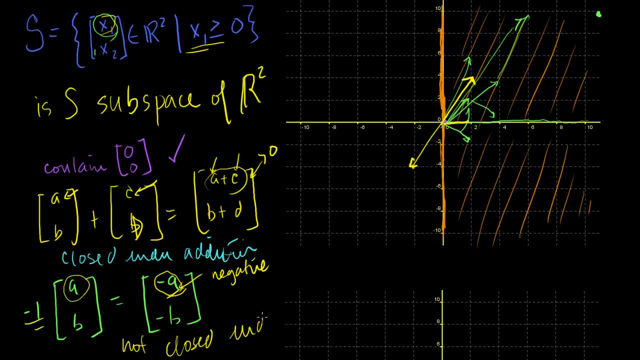 scalar multiplication Not closed. under scalar multiplication: Not closed. So this is not a subspace of R2.. Now I'll ask you one Interesting question. What if I ask you just the span of some set of vectors? Is that a valid 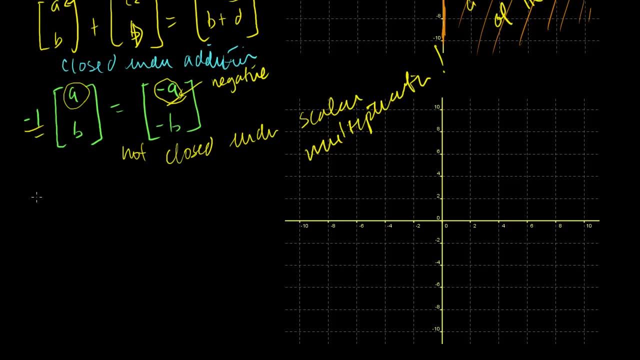 Let's say I have the span of some. Let's say I want to know the span of. yeah, I don't know. Let's say I have vector v1,, v2, and v3. And I'll be. you know, I'm not even going to tell you how. 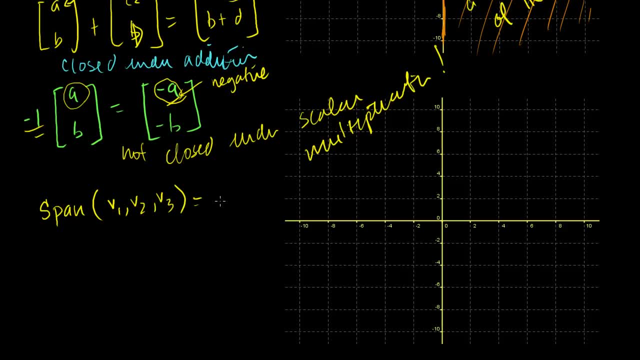 many elements each of these vectors have. Is this a valid subspace Of Rn, where, you know, n is kind of the number of elements that each of these have Of Rn. Well, let's pick one of the elements of. let me define, let 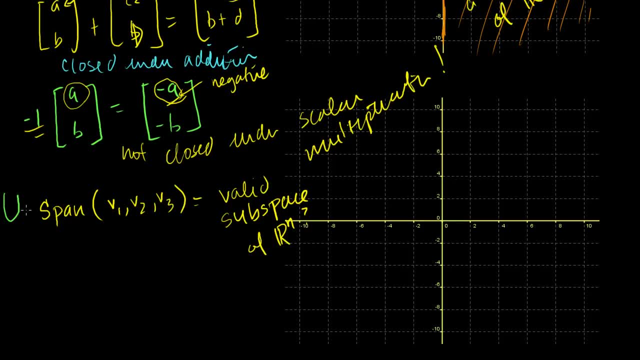 me just call u to be the set, or the set of all linear combinations of this is the span. So let me just define u to be the span. So I want to know: is u a valid subspace? So let's think about it this way. 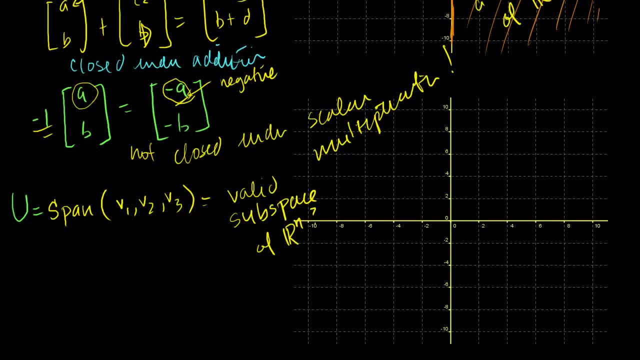 Let me just Pick out a random element of u. Let me pick out a random element of u. Actually, does this contain the 0 vector? Well, sure, If we just multiply all of these times 0, so if we just 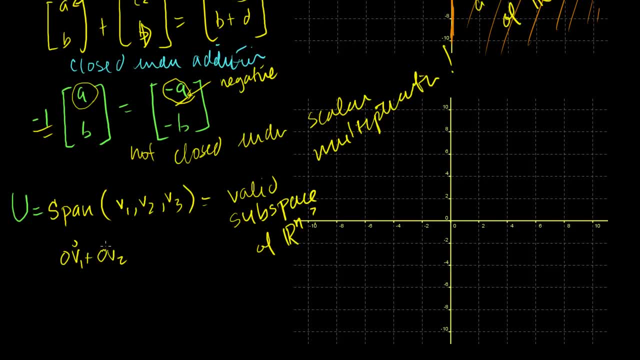 say: 0 times v1 plus 0 times v2, these are all vectors, I didn't write them bold- Plus 0 times v3, we get the 0 vector right. Everything just is zeroed out. So it definitely contains the zeroed vector. 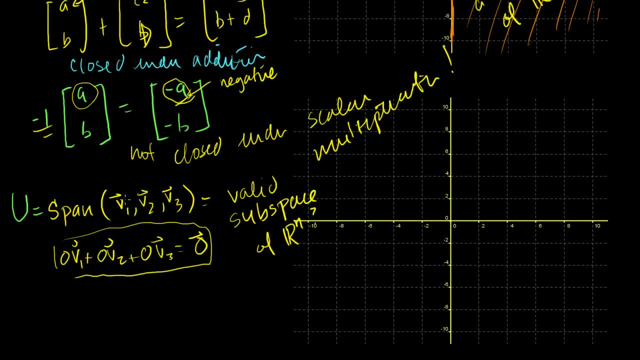 This is a linear combination of those three vectors, So it's included in the span. Now, what if I let me just pick some arbitrary member of this span? So, in order to be a member of this set, it just means that you can be represented. 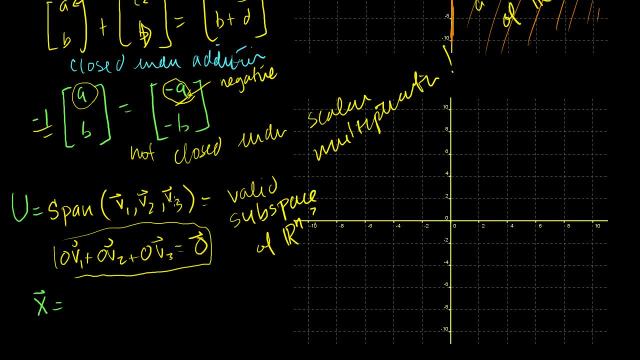 Let me just call the vector x. It means that you can be represented as a linear combination of these vectors, So some combination: c1 times v1 plus c2 times v2 plus c3 times v3.. Right, OK, OK, OK. 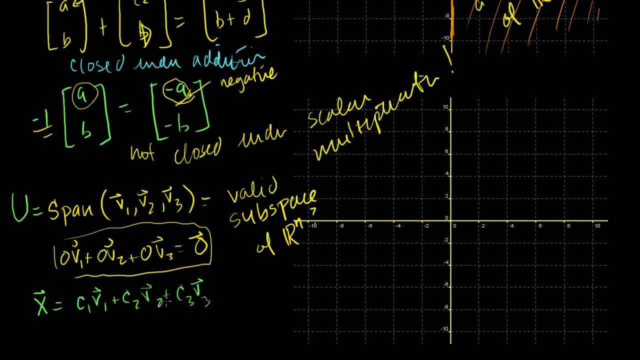 OK, OK, OK, OK, I'm just representing this vector x. It's a member of this, so it can be represented as a linear combination of those three vectors. Now is this set closed under multiplication? Well, let's just multiply. this times some arbitrary constant. 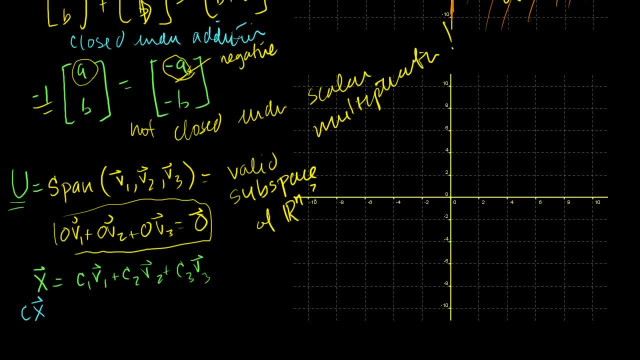 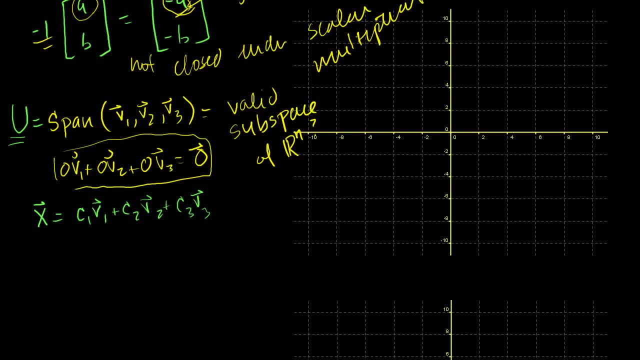 What is c times x? Let me scroll down a little bit. What is c times x equal? Let me do a different constant. actually, Let me multiply it times some arbitrary constant, a. What is a times x? Well, it's a times c1.. 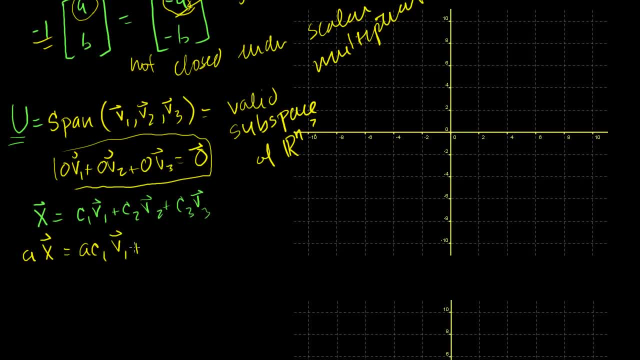 It's a times v1.. I'm just multiplying both sides of this equation: times a, a times c2, times v2 plus a times c3, v3.. Right, Well, you could just. I mean, if this was an arbitrary constant, you could just write this as another arbitrary. 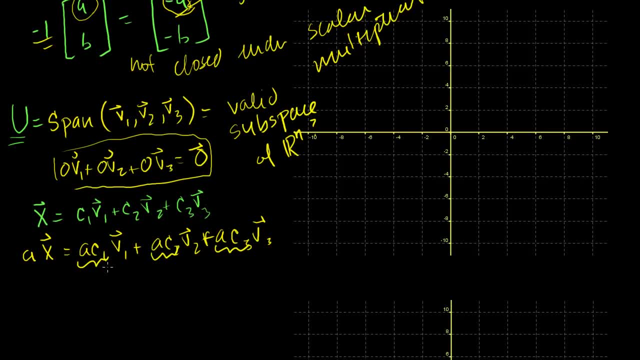 constant. this is another arbitrary constant. and this is another arbitrary constant And I want to be clear. All I did is I just multiplied both sides of this equation times a scalar, But clearly this expression right here, I mean I could. 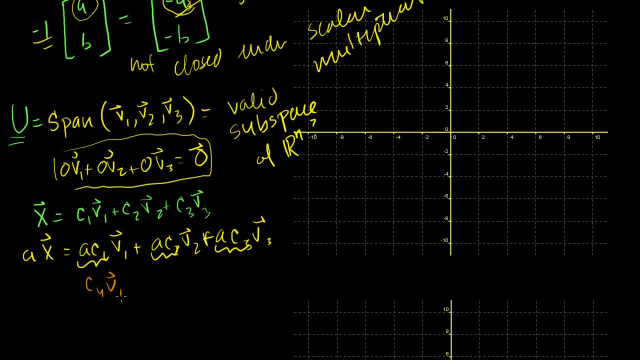 write this. I could rewrite this as you know, c1. So c4 times v1 plus c5 times v2, where this is c5, this is c4, plus c6 times v3. This is clearly another linear combination of these three. 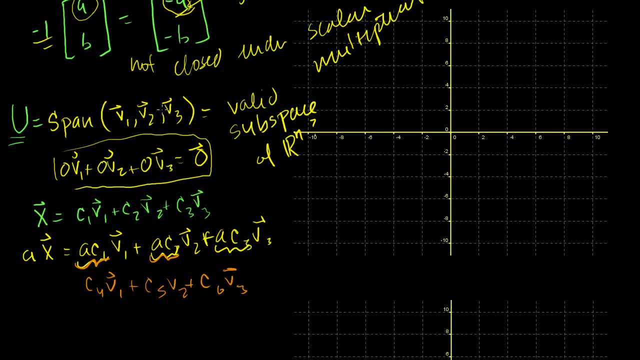 vectors. so the span is the set of all of the linear combinations of these three vectors. So clearly this is one of the linear combinations, so it's also included in the span. So this is also in u, It's also in the span of those three vectors. 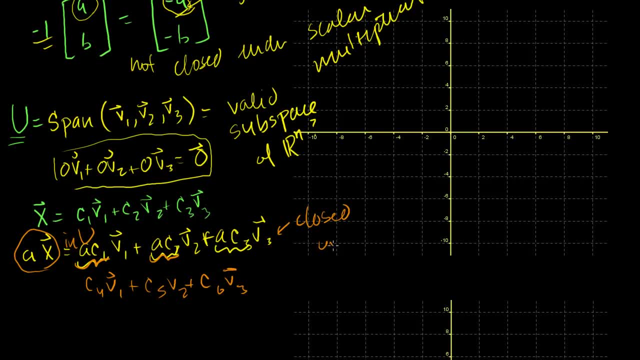 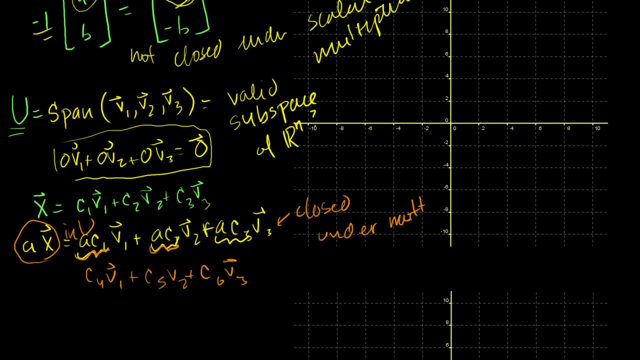 So it is closed, Closed under multiplication. Now we just have to show that it's closed under addition, and then we know that the span of- and we added 3 here, but you can extend it to an arbitrary n number of vectors- that the 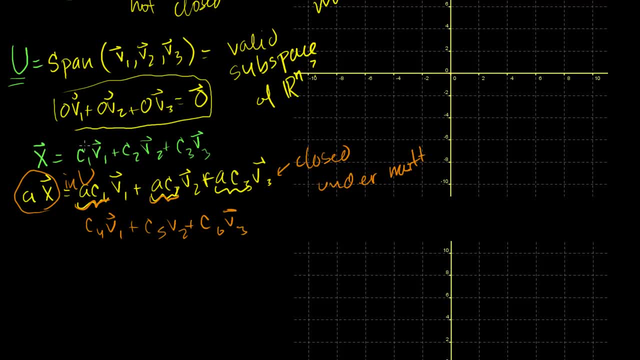 span of any set of vectors is a valid subspace. So let me prove that. So we already defined one x here. Let me define another vector that's in u or that's in the span of these vectors, And it equals, I don't know. 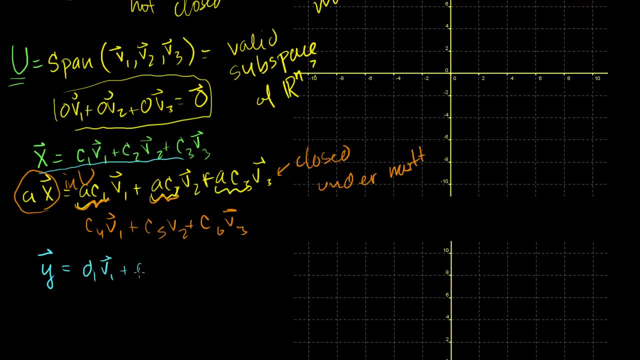 Let's say it equals d1 times v1, plus d2 times v2, plus d3 times v3.. Now what is x plus y? If I add these two vectors, what are they equal to? Well, I could just add: 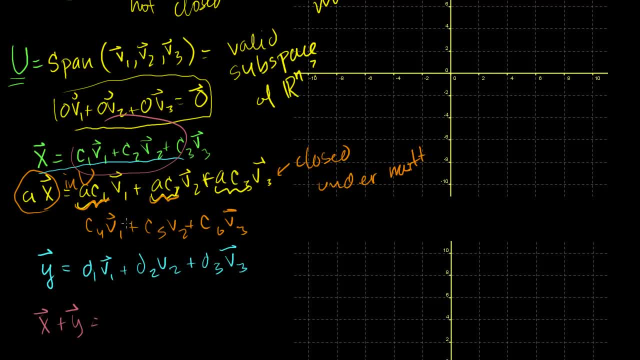 x plus y means all of this stuff plus all of this stuff. And so what does that equal? It means, if you just add these together, You get c1 plus d1 times v1, plus c2 plus d2 times v2, plus. 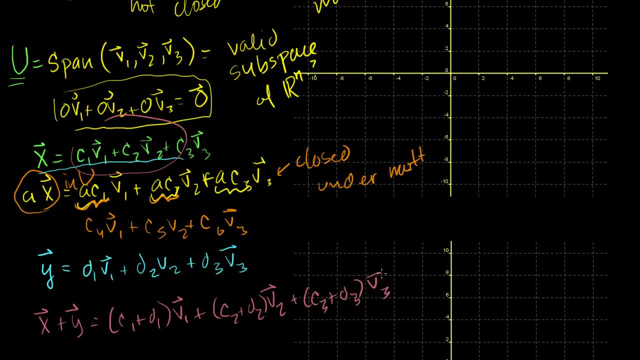 c3 plus d3 times v3.. You had a v3 here, you had a v3 there. You just add up their coefficients. Clearly this is just another linear combination. These are just constants. again, That's an arbitrary constant. 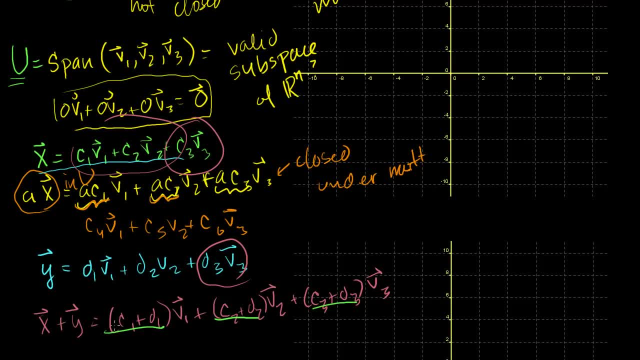 That's an arbitrary constant. That's an arbitrary constant. So this thing is just a linear combination. It's a linear combination of v1, v2, and v3.. So it must be, by definition, in the span of v1, v2, and v3.. 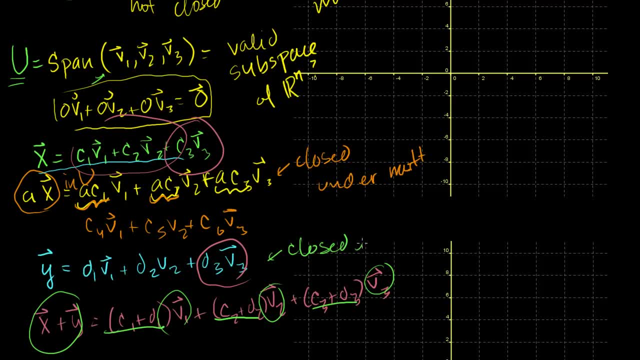 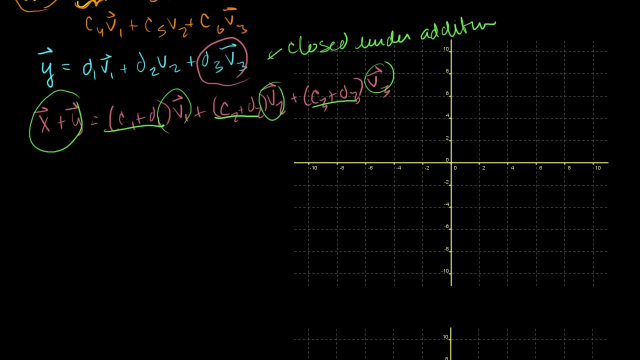 So we are definitely closed. under addition. Now you might say: hey, Sal, you're saying that the span of any vector is a valid subspace. But let me show you an example that clearly, if I just took the span of one vector, 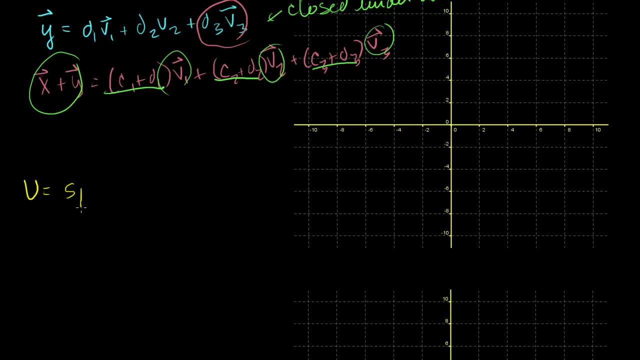 Let me just say: Let me just define u to be equal to the span of just the vector. let me just do a really simple one. Let's say it's just the vector 1, 1.. Clearly this can't be a valid subspace. 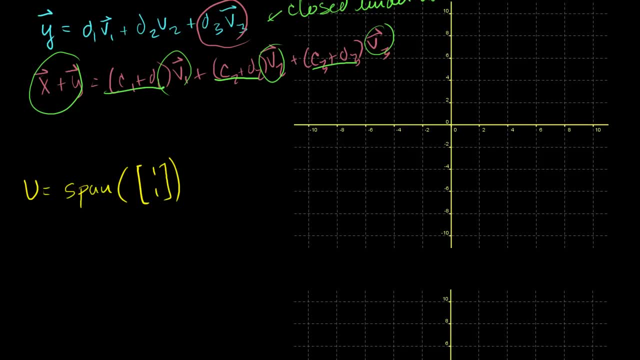 Let's think about this visually. So what does a vector 1, 1 look like? Vector 1, 1 looks like this And the span of vector 1, 1 is all of, and this is in its standard position. the span of vector 1, 1 is all of the. 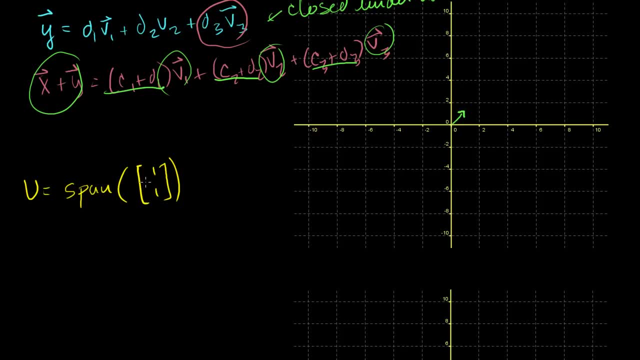 linear combinations of this vector. Well, there's nothing else to add it to, So it's really just going to be all of the scaled up and scaled down versions of this. So if you scale it up, you get things that look more like: 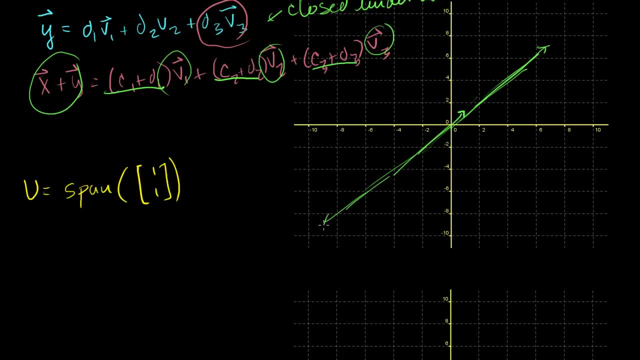 that if you scale it down, you get things that look more like that if you go into the negative domain. So just by multiplying this vector times different values, and if you were to put them all into a standard position, you would essentially get a line that looks like that: 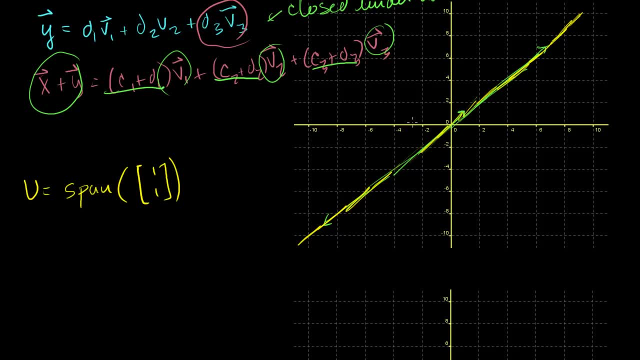 You say, gee, that doesn't look like a whole subspace. But a couple of things. clearly, it contains the vector 0, 1, 0,. it contains the 0 vector. We can just scale it by 0.. 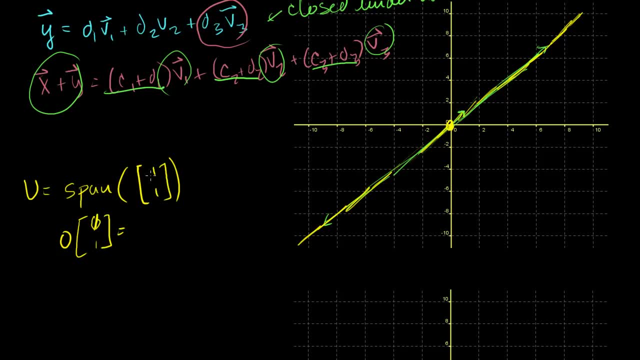 The span is just all of the different scales of this, And if there were other vectors, you would add it to those as well, But this is clearly going to be the 0 vector, So it contains the 0 vector. Is it closed? under multiplication. 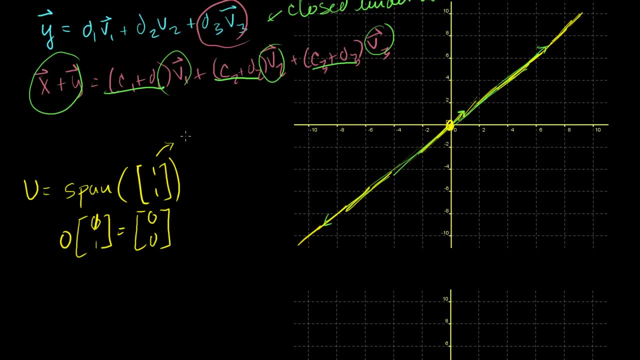 Well, the span is the set of all of the vectors where, if you take all of the real numbers for c and you multiply it times 1, 1, that is the span. So clearly you multiply this times anything it's going to. 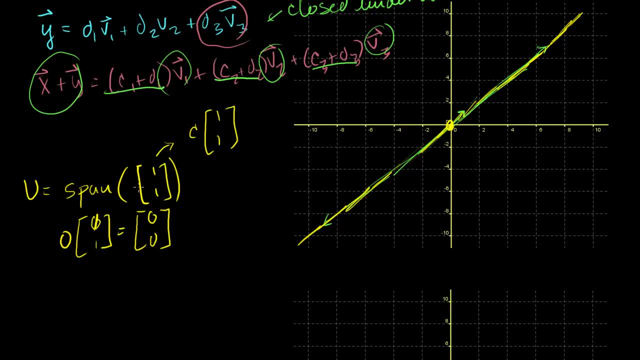 equal. another thing that's definitely in your span. Now the last thing, is it closed under addition? So any two vectors in the span could. let's say that I have one vector a that's in my span. I can represent it as c1, some scalar times my vector there.